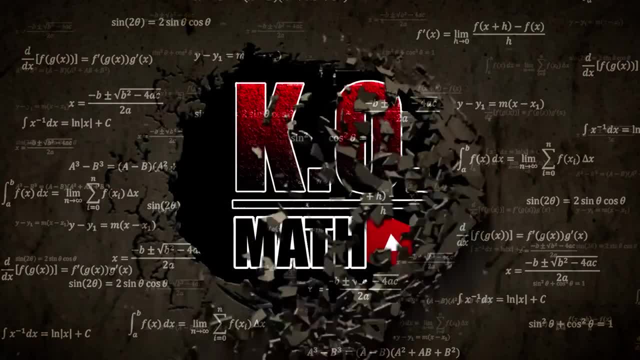 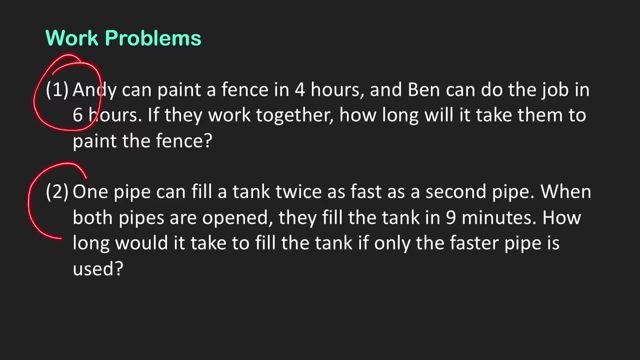 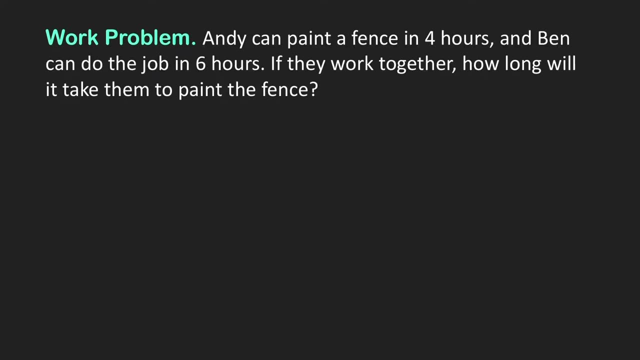 In this video we're going to solve these two work problems, and these are applications of linear equations. Let's get started. First problem: Andy can paint a fence in four hours and Ben can do the same job in six hours. If they work together, how long will it take them to paint the fence? 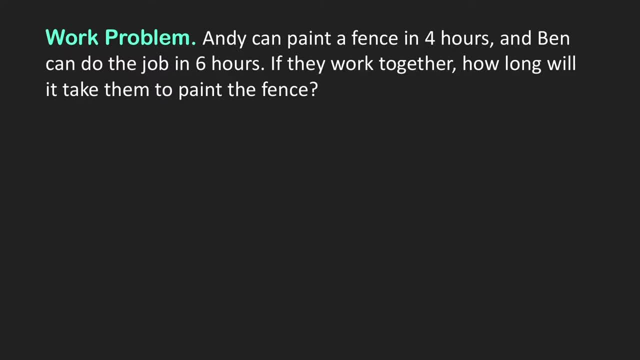 So how do we solve this problem? We can easily set up our model or our equation that will solve this problem if we know the following: If it takes n units of time to do a job, then 1 over n of the job is completed per unit of time. This means that if you can do a job in four days, then you can. 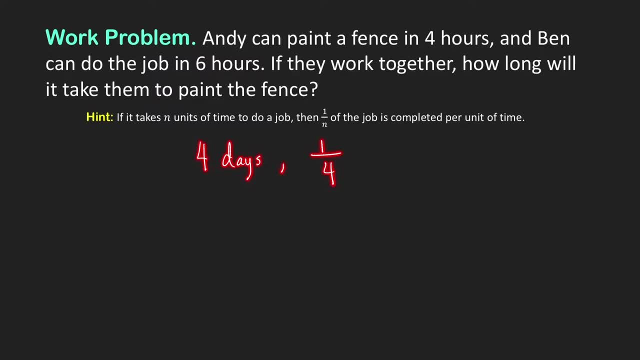 complete 1 over 4 of the job, one fourth of the job per day, which makes sense, And if you can do the job, let's say in 10 days, then this means that you can complete 1 over 10, or one tenth of. 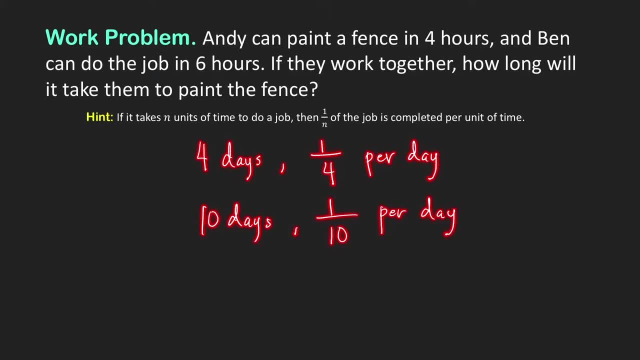 the job per day. So if you can do the job in four hours, then you can complete one fourth of the job per hour, and so on. So if it takes n units of time to do a job, then we are sure that 1 over. 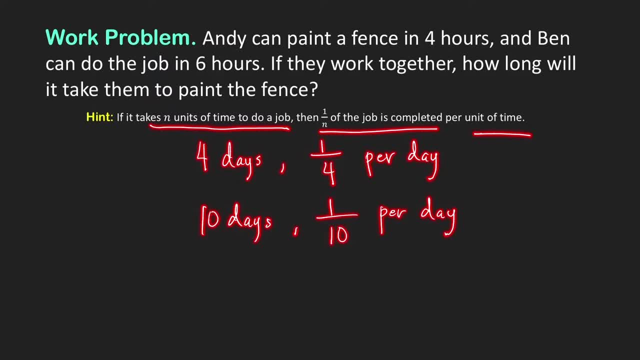 n of the job is completed per unit of time, And your unit of time could be minute, hour, day, month and so on. Let's now solve our problem. Using this hint here, we can easily set up our equations that will solve this kind of work problems. So for this problem, it says that: 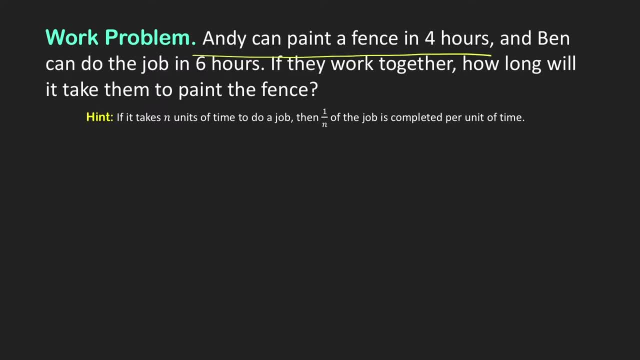 Andy can paint a fence in four hours, which means that Andy can complete one fourth of the job in one hour. So let's write that down. So this is for Andy, And let's write down the time It takes Andy to complete the job, and that is. 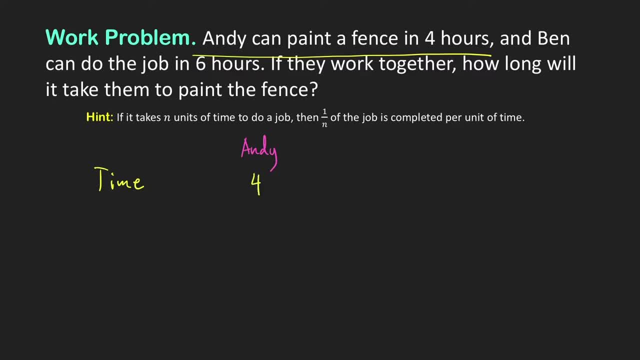 four hours, So this is equal to four. And here it says that Ben can do the job in six hours, So let's write down that time. So Ben here takes six hours to complete the job. And what are we looking for? We're looking for the time it takes them to paint the fence. 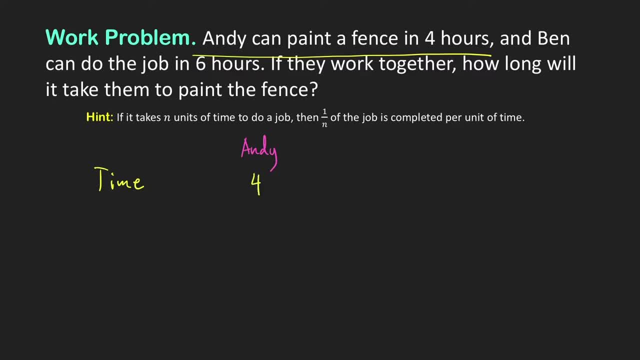 four hours, So this is equal to four. And here it says that Ben can do the job in six hours, So let's write down that time. So Ben here takes six hours to complete the job. And what are we looking for? We're looking for the time it takes them to paint the fence. 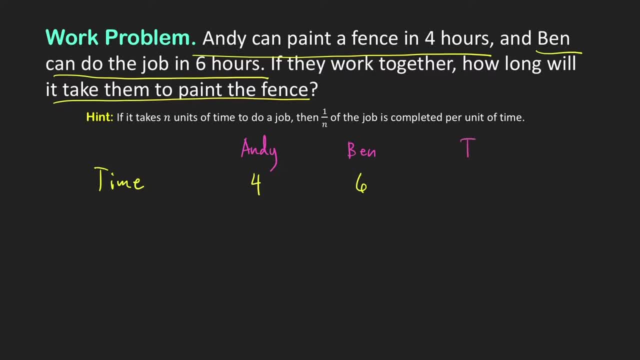 So this is unknown. So we can represent that by a variable. Let's say using x, So working together. let's say that it takes them x hours to complete the job And from this information we can now find the work done in one hour using this hint here. So if we compute for the work, 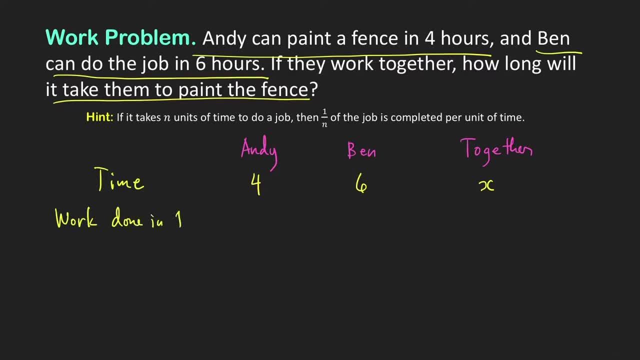 done in one hour. we can now find the work done in one hour. So if we compute for the work done in one hour, then since Andy can complete the job in four hours, then he can finish one fourth of the job in one hour. And how about Ben? Since Ben can do the job in six hours, then Ben can do one over. 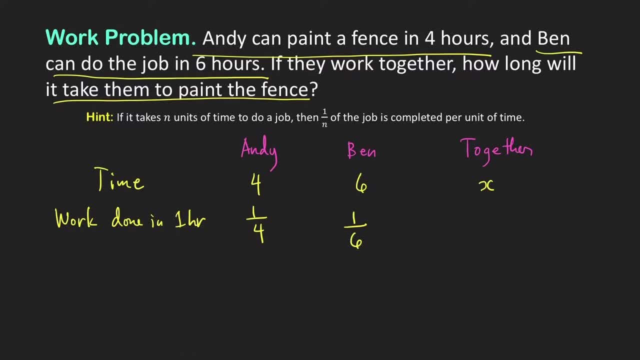 six of the job in one hour. Similarly, if they can finish the job in x hours, then they can do one over x of the job. So the work done in one hour by both is equal to one over x, And from this we can easily obtain: 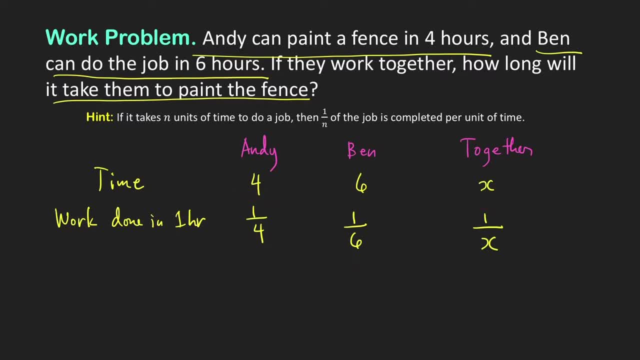 our equation, because we know that if we add the work done by Andy and Ben, it should be equal to the work done by both, which is equal to one over x. Therefore, this is a model for our problem And for sure you can easily solve this equation here. 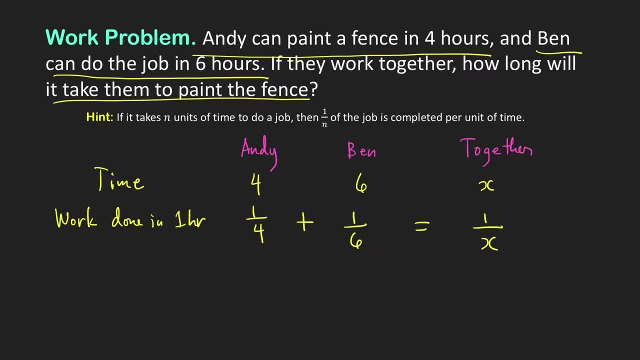 How do we solve this equation? So to solve this equation we can multiply both sides by the LCD to get rid of the denominators. And the LCD here is 12x. So we can do 12x times one over four, and then plus one over six, equal to one over x times 12x, And this will get rid of all the denominators. 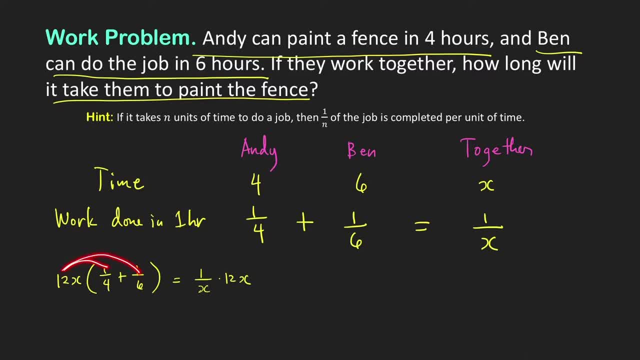 and we'll get an equation. So we have to distribute this to each term in this grouping symbol. So we get here 12x over four, So that is equal to 3x, and then plus 12x over six, So that is equal. 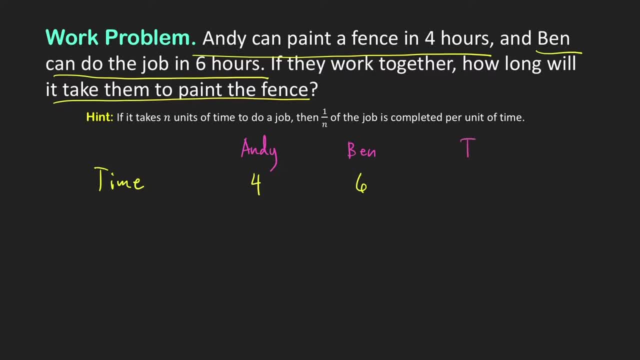 So this is unknown. So we can represent that by a variable. Let's say using x, So working together. let's say that it takes them x hours to complete the job And from this information we can now find the work done in one hour using this hint here. So if we compute for the work, 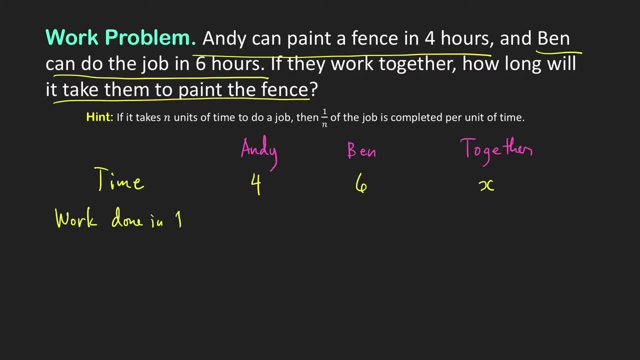 done in one hour. we can now find the work done in one hour. So if we compute for the work done in one hour, we can now find the work done in one hour. So if we compute for the work done in one hour, 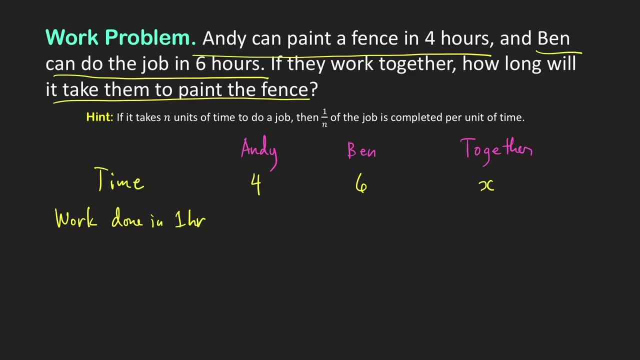 then, since Andy can complete the job in four hours, then he can finish one fourth of the job in one hour. And how about Ben? Since Ben can do the job in six hours, then Ben can do one over six of the job in one hour. Similarly, if they can finish the job in x hours, then they can do one. 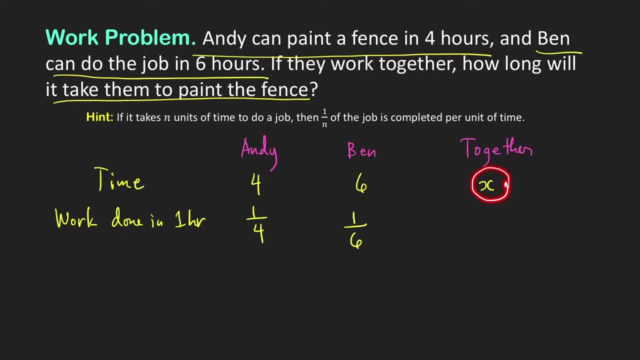 over x of the job. So the work done in one hour by both is equal to one over x, And from this we can easily obtain our equation, because we know that if we add the work done by Andy and Ben it should be equal to. 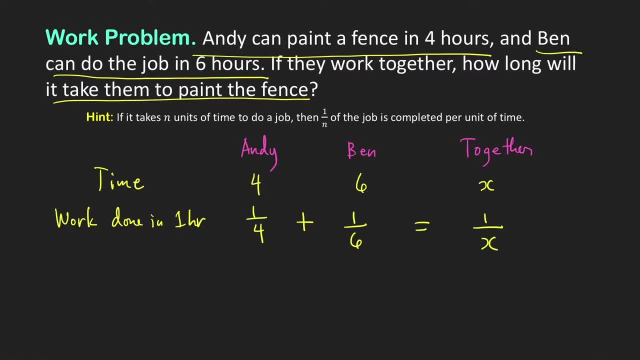 the work done by both, which is equal to one over x. Therefore, this is a model for our problem And for sure you can easily solve this equation here. How do we solve this equation? So to solve this equation, we can multiply both sides by the LCD. 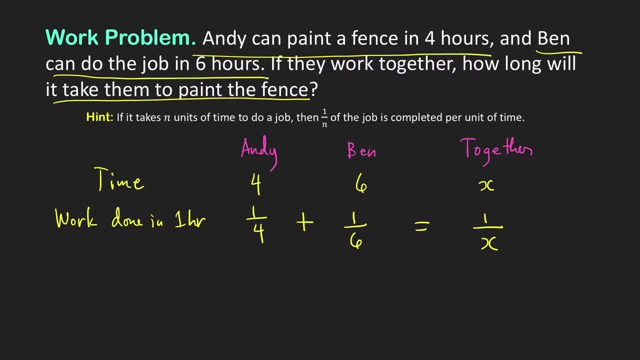 to get rid of the denominators And the LCD here is 12x, So we can do 12x times one over four and then plus one over six, equal to one over x times 12x, And this will get rid of all the denominators. 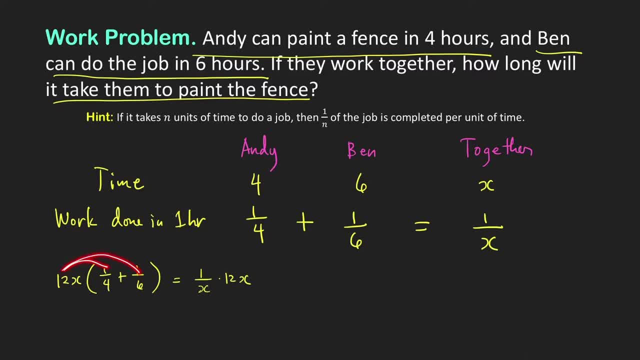 and we'll get an equation. So we have to distribute this to each term in this grouping symbol. So we get here 12x over four, So that is equal to 3x, and then plus 12x over six, So that is equal. 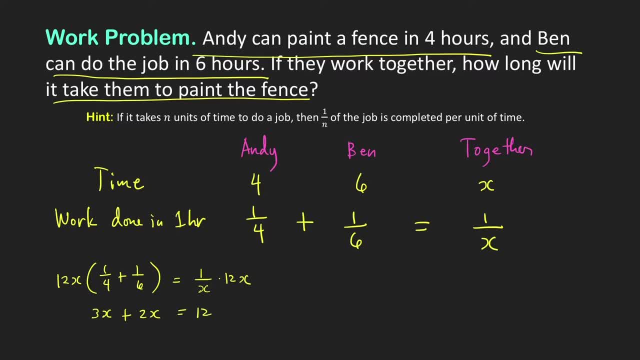 to 2x, which is equal to 12.. And this will give us 5x equal to 12.. So, therefore, x is equal to 12 over five, which is equal to 2.4.. And the unit is hours, And this is equal to two hours, and. 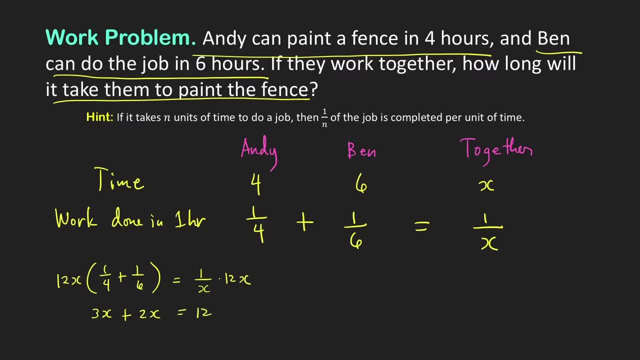 to 2x, which is equal to 12.. And this will give us 5x equal to 12.. So, therefore, x is equal to 12 over five, which is equal to 2.4.. And the unit is hours, And this is equal to two hours, and. 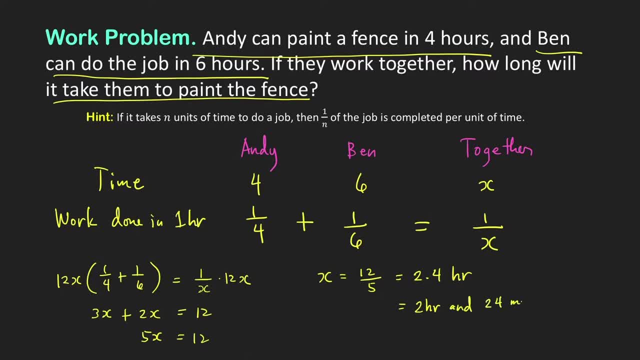 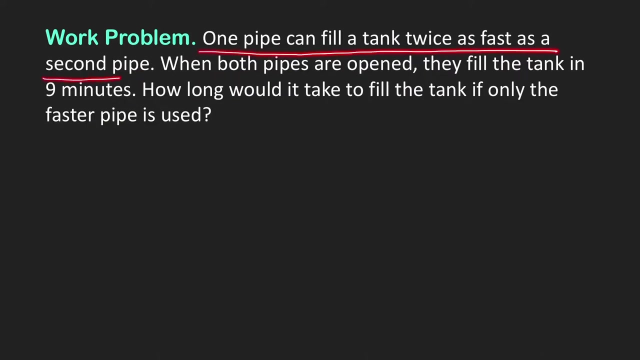 how many minutes? 24.. 24 minutes, And this is already the answer to our problem. This means that if they work together, they need two hours and 24 minutes to paint the fence. Now let's move to the second problem. One pipe can fill a tank twice as fast as a second pipe. 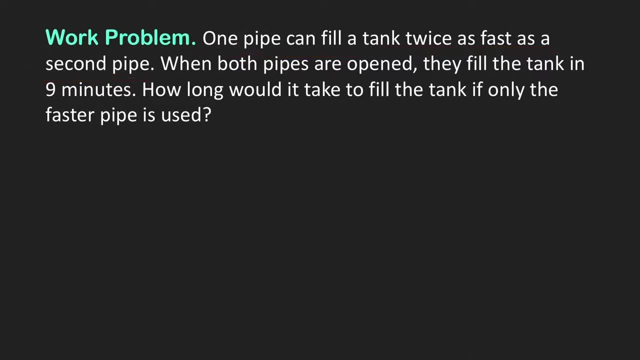 When both pipes are opened, they fill the tank in nine minutes. How long would it take to fill the tank if all pipes are open? How long would it take to fill the tank if all pipes are open, only the faster pipe is used. so we apply the same strategy to solve. 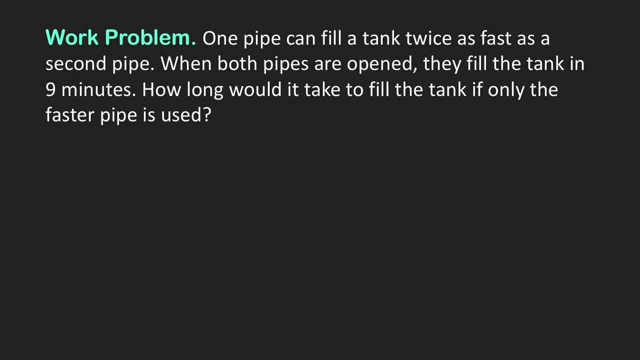 this problem. so here we have two pipes, so we have this lower pipe and the faster pipe. now what is the time that it takes for each pipe to fill the tank? so here we don't know the exact time for each pipe to fill the tank. however, we know from this information that one pipe can fill the tank twice, as 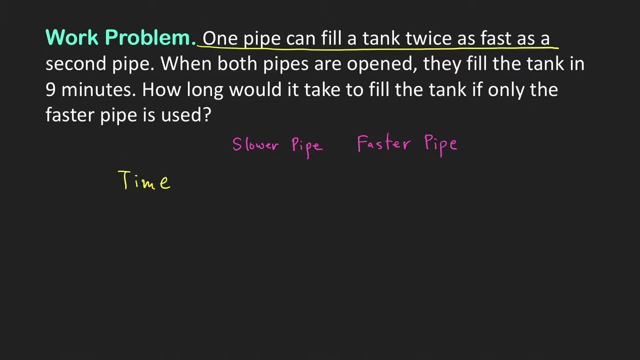 fast as the other. this means that if the slower pipe can fill the tank in four hours, then the faster pipe can fill the tank in just two hours. why? because this faster pipe can fill the tank in two hours and the slower pipe can fill the tank twice as fast. 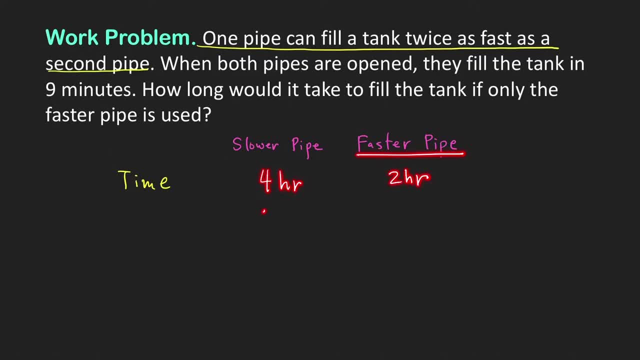 as the slower pipe. so if the slower pipe can do the job in eight hours, then we are sure that the faster pipe can do the job in just half of that, which is four hours. so this means that the time for the faster pipe is just half of the time of the slower pipe. so if we let 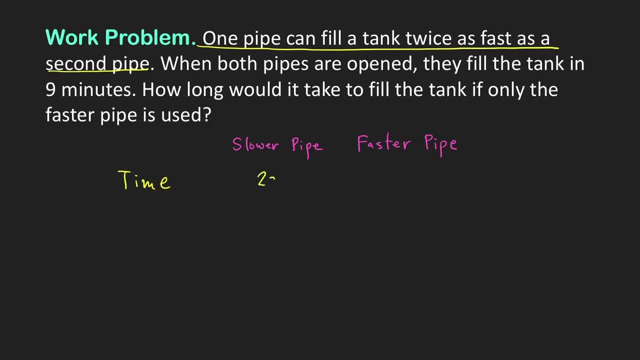 the time for this lower pipe to be equal to, let's say, 2x, then the time for the faster pipe is just half of this, which is 2x over 2, so that is equal to x. now from the second sentence we know that when both pipes are opened, 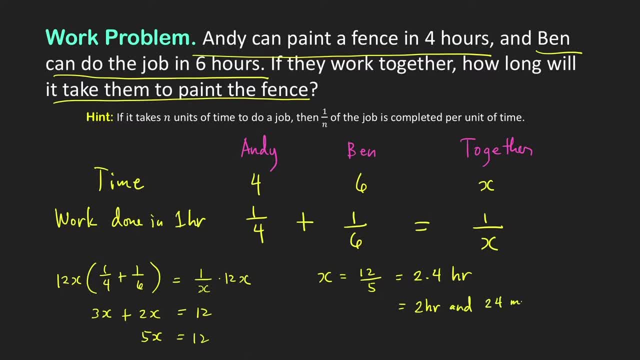 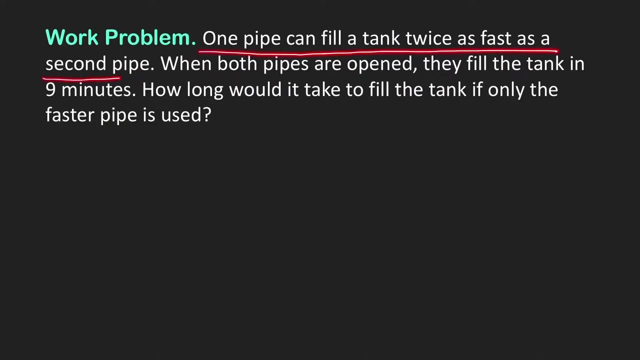 how many minutes? 24 minutes, And this is already the answer to our problem. This means that if they work together, they need two hours and 24 minutes to paint the fence. Now let's move to the second problem. One pipe can fill a tank twice as fast as a second pipe, When both pipes are opened. 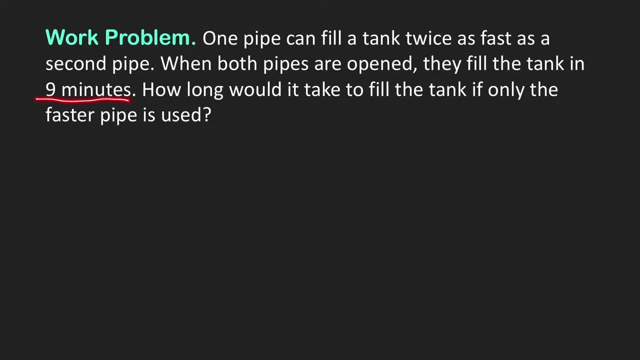 they fill the tank in nine minutes. How long would it take to fill the tank if only the faster pipe is used? So we apply the same strategy to solve this problem. So here we have two pipes, so we have the slower pipe and the faster pipe. 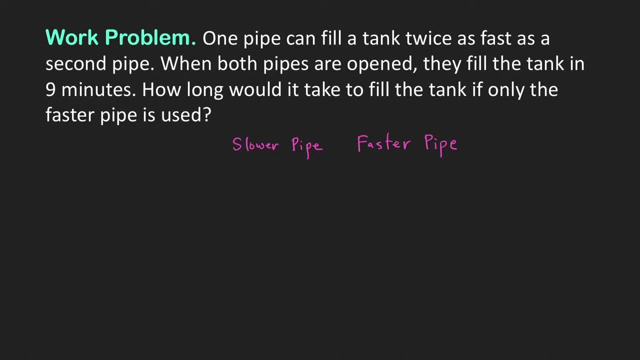 Now, what is the time that it takes for each pipe to fill the tank? So here we don't know exact time for each pipe to fill the tank. however, we know from this information that one pipe can fill the tank twice as fast as the other. this 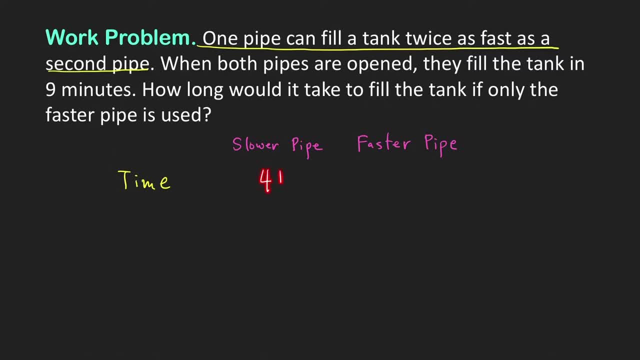 means that if the slower pipe can fill the tank in four hours, then the faster pipe can fill the tank in just two hours. why? because this faster pipe can fill the tank twice as fast as the slower pipe. so if the slower pipe can do the job in eight hours, then we are sure that the faster pipe can do the job in just 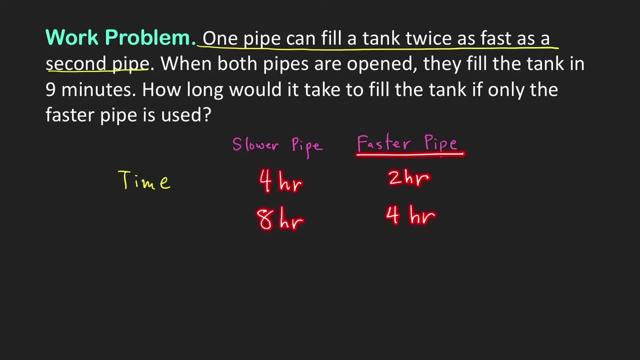 half of that, which is four hours. so this means that the time for the faster pipe is just half of the time of the slower pipe. so if we let the time for the slower pipe to be equal to, let's say, 2x, then the time for the faster pipe is. 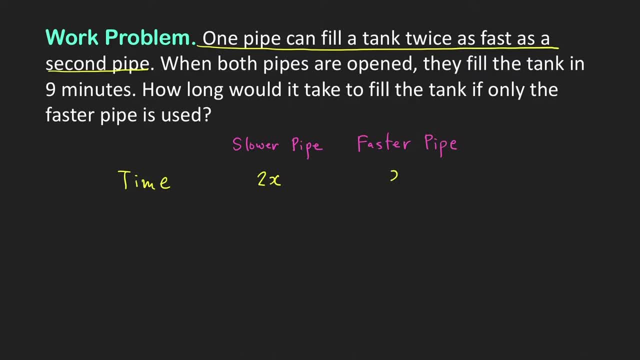 just half of this, which is 2x over 2, so that is equal to X. now from the second sentence we know that when both pipes are opened they fill the tank in nine minutes. so this is the together time, so together they can do the job in nine. 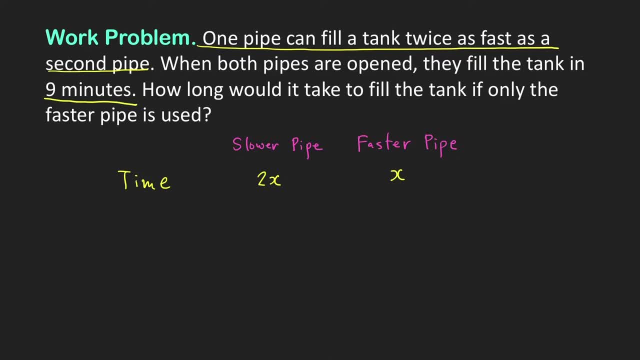 they fill the tank in nine minutes. so this is the together time, so together they can do the job in nine minutes. now that we already know these times, we can now find the work done in each unit of time, so in this case, work done in one minute. 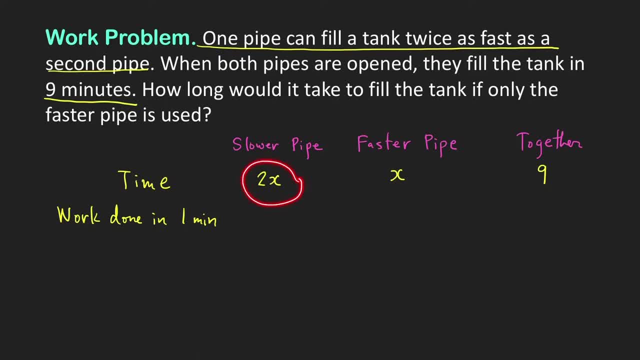 so if the slower pipe can fill the tank in two x minutes, then this pipe can fill one over two x. again, we use the same strategy as what we used in the first problem, and since the faster pipe can fill the tank in x minutes, then this in x minutes, then this pipe can fill one over x of the tank in one minute. 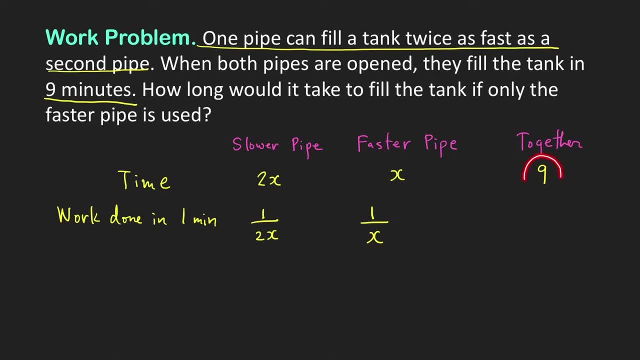 and since the two pipes can fill the tank in nine minutes, then this means that they can fill one over nine of the tank in one minute, and from this we obtain our equation: one over two, x plus one over x is equal to one over nine. and again, to solve this equation we first multiply by the lcd, and the lcd here is 18x. 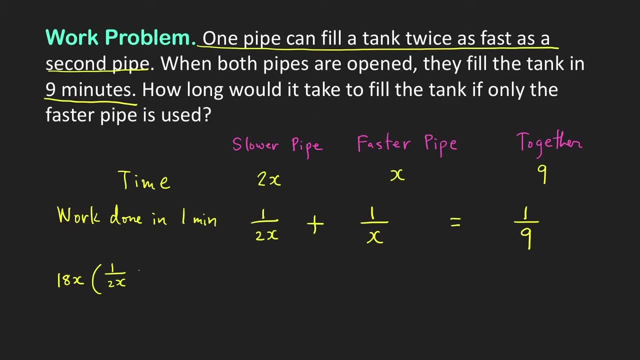 so we have here 18x times one over two x plus one over x, equal to one over nine times 18x, which gives us nine plus 18x equal to 2x, which is equivalent to 27 equal to 2x. so therefore, our x is equal to 27 over 2. 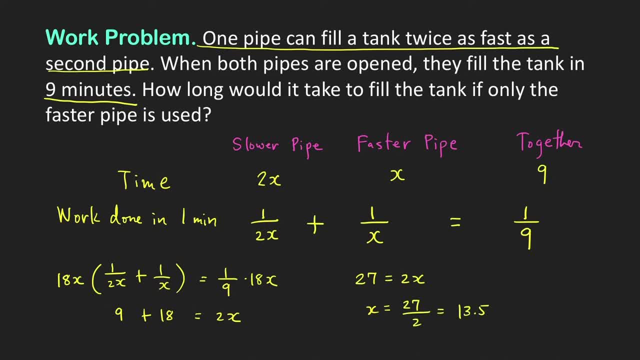 which is equal to 13.5. and what is the unit of x? it is in minutes. so now what is the answer to our problem? since we're asked to find the time, it takes four minutes for the faster pipe to fill the tank alone, and we let this time to be x. therefore, the answer is 13.5 minutes. 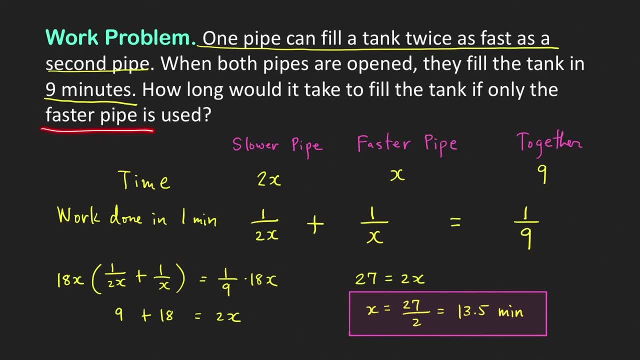 if, instead of the faster pipe, we are asked to find the time it takes for the slower pipe to fill in the tank, then our answer will be the value of 2x, which is in this case equal to 27 minutes. so make sure to answer what is being asked in the problem when you're solving word problems. 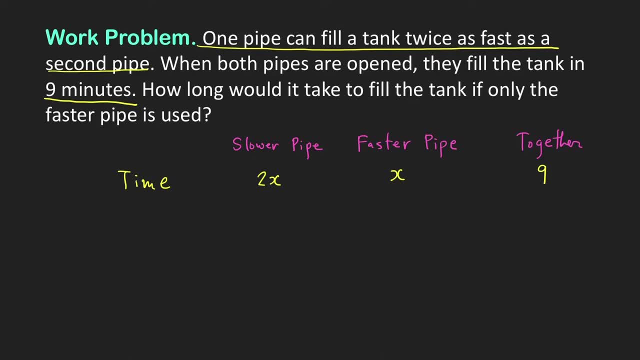 minutes. now that we already know these times, we can now find the work done in work done in each unit of time. so in this case work done in one minute. so if the slower pipe can fill the tank in 2x minutes, then this pipe can fill one over 2x again. we 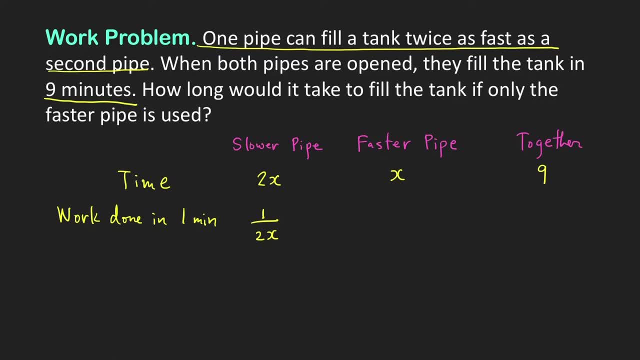 use the same strategy as what we used in the first problem, and since the faster pipe can fill the tank in X minutes, then this pipe can fill one over X of the tank in one minute. and since the two pipes can fill the tank in nine minutes, then this means that they can fill one over nine of the tank in. 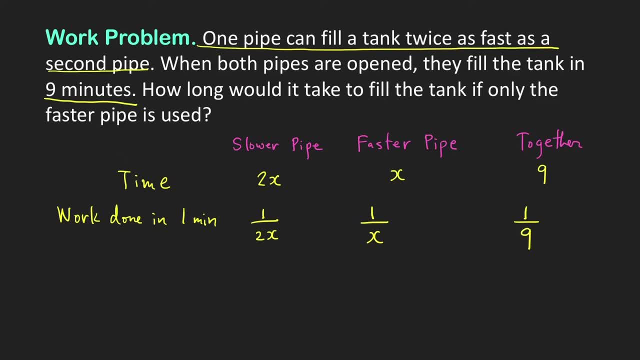 one minute and from this we obtain our equation: 1 over 2x plus 1 over X is equal to 1 over 9. and again, to solve this equation, we first multiply by the LCD, and the LCD here is 18 X, so we have here 18 X. 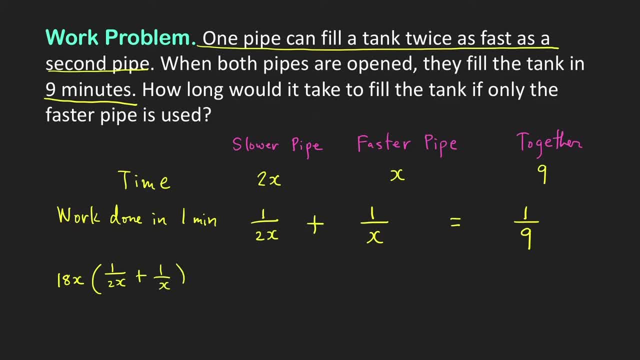 times 1 over 2 X plus 1 over X, equal to 1 over 9 times 18 X, which gives us 9 plus 18 equal to 2 X, which is equivalent to 27 equal to 2 X. so So, therefore, our x is equal to 27 over 2,, which is equal to 13.5.. 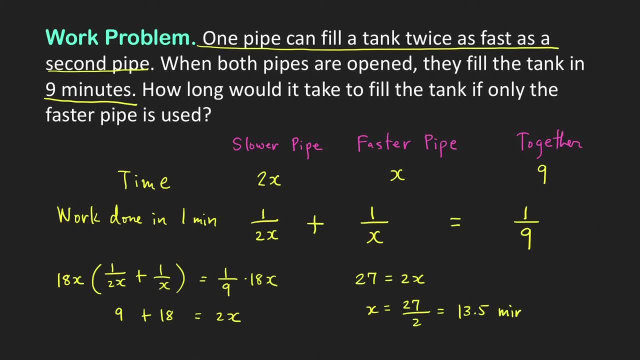 And what is the unit of x? It is in minutes. So now what is the answer to our problem, Since we're asked to find the time it takes for the faster pipe to fill the tank alone and we let this time to be x? 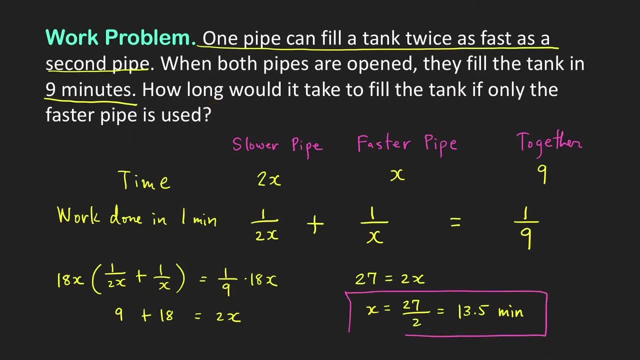 therefore, the answer is 13.5 minutes. If, instead of the faster pipe, we are asked to find the time it takes for the slower pipe to fill in the tank, then our answer will be the value of 2x, which is, in this case, equal to 27 minutes. 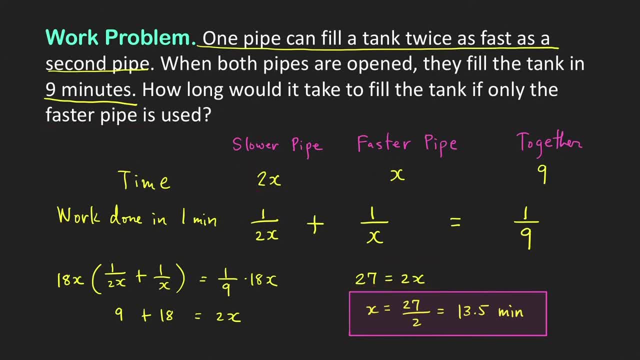 So make sure to answer what is being asked in the problem when you're solving word problems, because sometimes you might be asked to find the value of 2x instead of x. So the solution to your model or to your equation is not necessarily the answer to the problem.